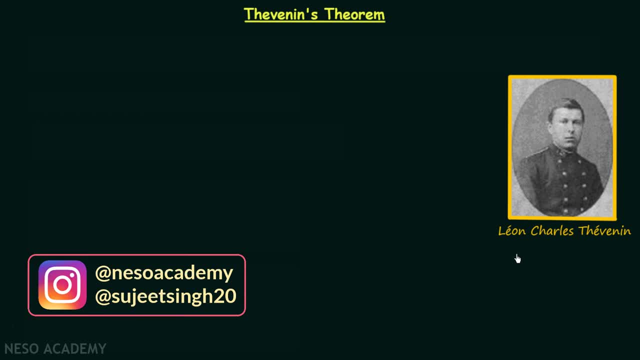 the equivalent circuit and the statement of the Thevenin's theorem, we will first understand why Thevenin's theorem is needed. It often happens that a particular element in a circuit is variable, while the other elements are fixed. Each time the variable element is changed, the entire. 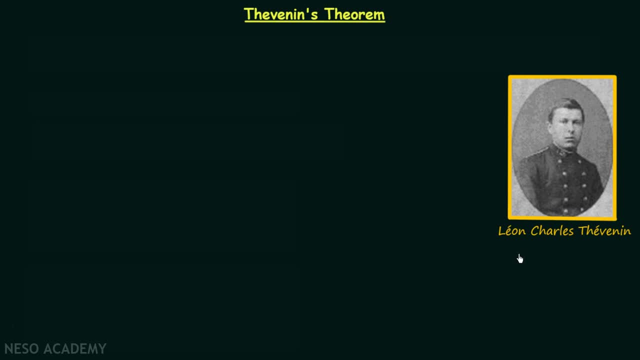 circuit has to be analyzed again To avoid this problem. Thevenin's theorem provides a technique by which the fixed part of the circuit is replaced by an equivalent circuit. So it is very easy to understand that In a lightweight circuit the على- melanin part of the circuit between the 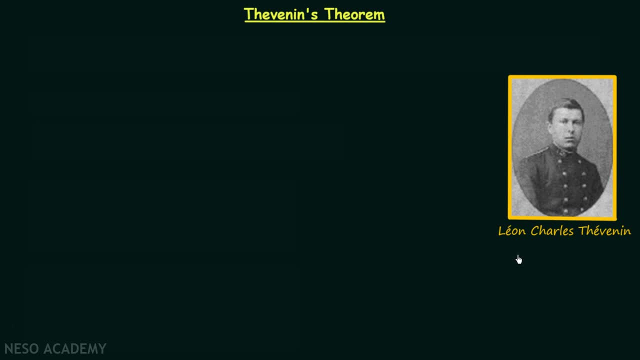 all- delineated wires judges is the same When divided into two eateries creating a, including electrical, large, complex network. there is one element which is variable, while the other elements are fixed, And when this variable element is changed, the analysis has to be done again. 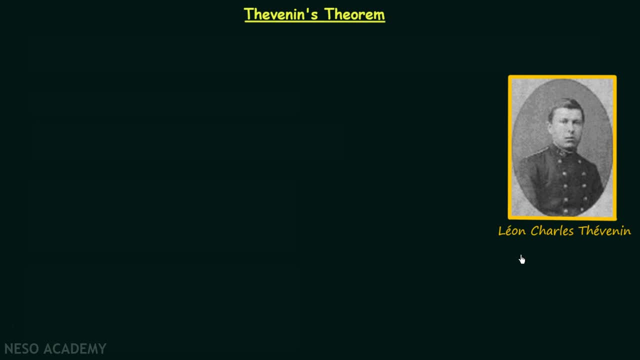 Now, to avoid this problem, we replace the fixed part of the circuit by the equivalent circuit, known as the Thevenin's equivalent circuit. And this equivalent circuit is very simple and therefore, when the variable part is changing, we do not have to perform the tedious calculations again. 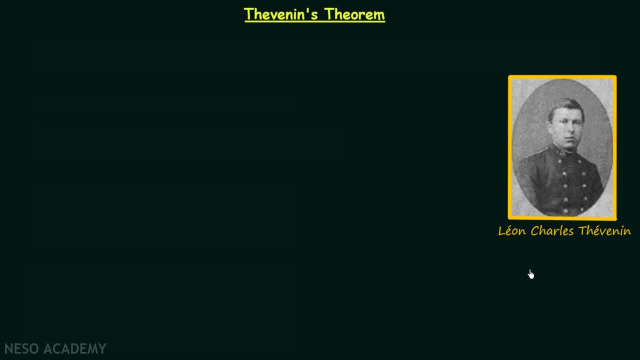 All these points will become crystal clear by the end of this lecture. Now we will move on to the statement of Thevenin's theorem. According to the statement, a linear bidirectional two-terminal network can be replaced by an equivalent network consisting of a voltage source- Vth- connected in series with a resistor. 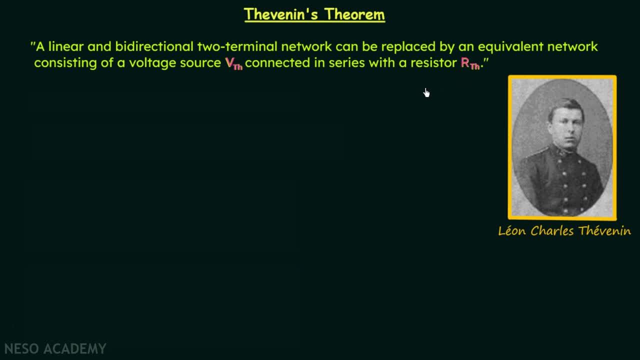 Rth. So, as I said earlier, Thevenin's theorem provides a technique By which we can replace the fixed part of the circuit by the equivalent circuit, and the equivalent circuit or network will have Vth connected in series with Rth. So you can think about the simplicity this theorem is providing. 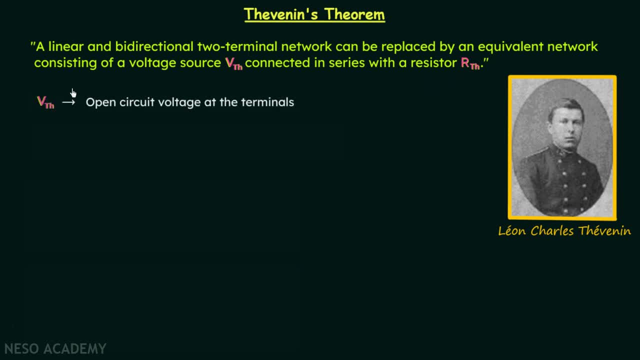 Now what is Vth and what is Rth? Vth, which is known as the Thevenin's voltage, is open circuit voltage at the terminals. We will understand how we can calculate Vth in the network. And Rth, which is known as the Thevenin's resistance, is the input or equivalent resistance. 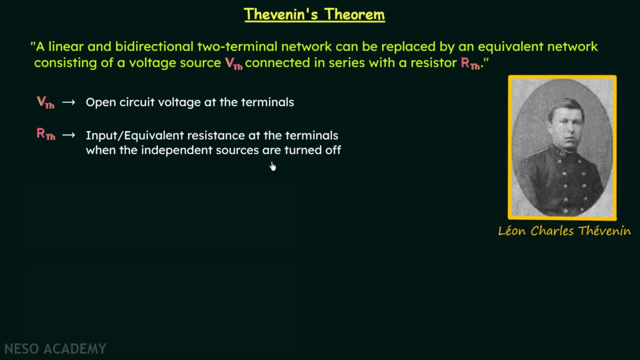 at the terminals when the independent sources are turned off, And we will understand how to calculate Vth and Rth by taking one example To summarize our discussion. till this point, I have taken this particular arrangement in which we have a linear and bidirectional network which is having fixed voltage. 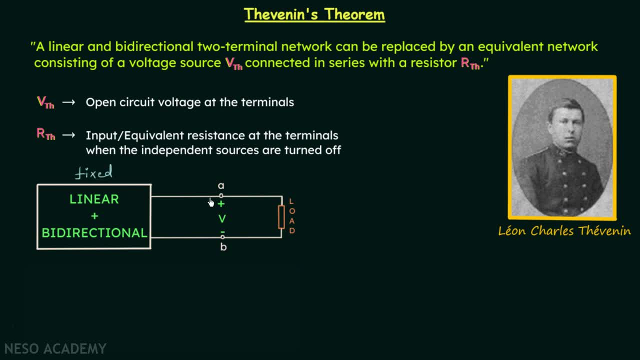 Fixed elements and from this network we are getting two terminals across which one load is connected, and this load is a variable load. And therefore, for the simplicity, it is good to have the Thevenin's equivalent circuit in place of this network, And we know what is Thevenin's equivalent circuit. 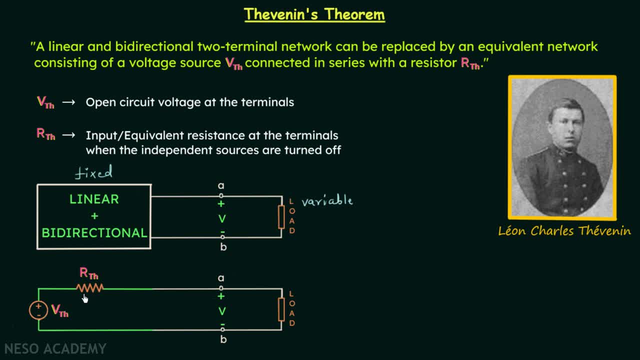 It is Vth connected in series with Rth. So here we have replaced this particular network By Vth connected in series with Rth. Now the only problem is we don't know how to find out Vth and how to find out Rth. 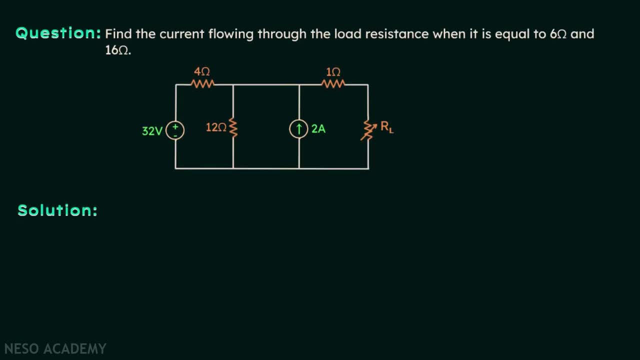 For this, I have taken one example in which we are required to find out the current flowing through this load resistor, which is variable in nature, when it is equal to 6 ohms and it is equal to 16 ohms. I want you to analyze the given circuit for some time, and then we will move on to the 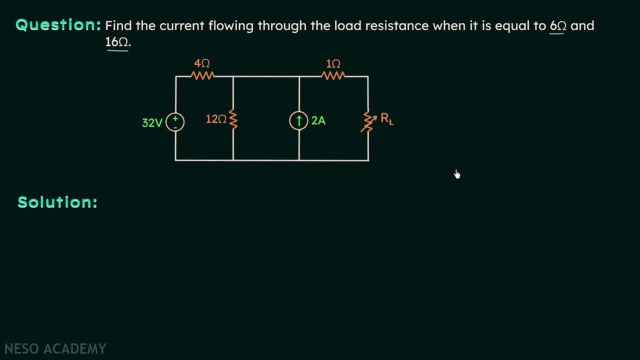 solution. I hope you are done. Now. we will move on to the calculation of current flowing through RL when it is equal to 6 ohms and it is equal to 16 ohms, And to find out the current, we will first find out the Thevenin's equivalent circuit. 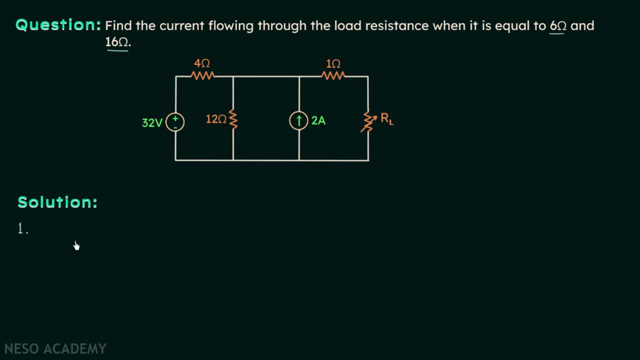 And we know, to find out Thevenin's equivalent circuit we need Vth and we need Rth. So first we will find out Thevenin's voltage Vth. For this purpose we will make one modification in our network And the modification is: we will remove the load resistance and we will open circuit the 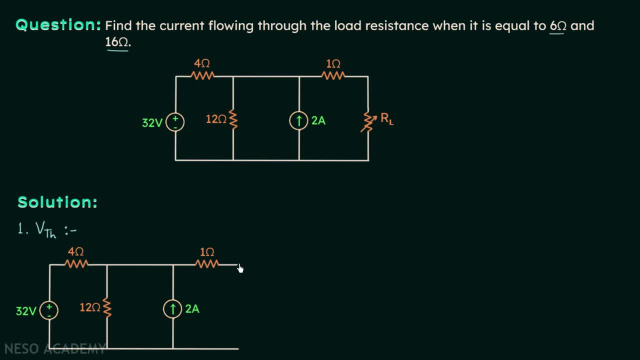 branch like this, And we are doing this because Vth is the open circuit voltage between these two terminals. And remember one thing: Always, Always, take the polarity like this and keep the polarity like this in the equivalent circuit as well. Do not reverse the polarity in the equivalent circuit. 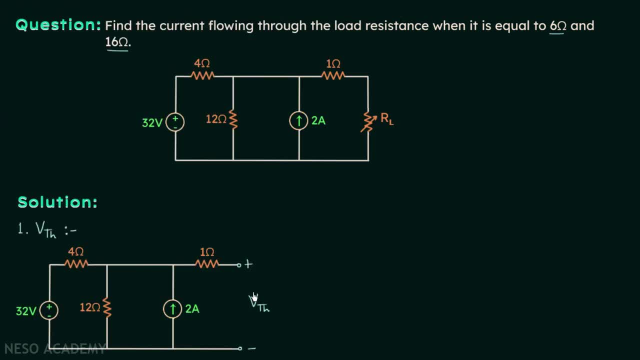 Keep it like this. Now we will find out Vth in this modified network. If we talk about the current flowing in this branch, then it will be zero. Why? Because this branch is open circuited And, if I assume, the potential at this node, 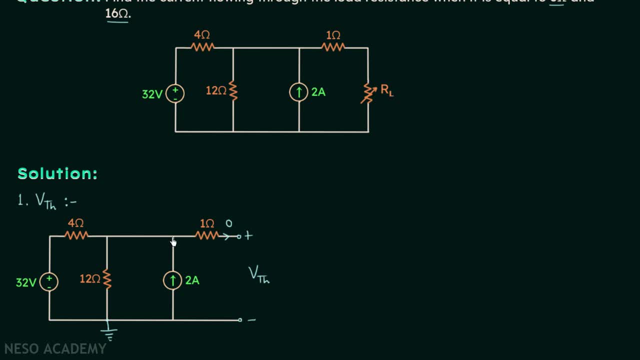 Equal to zero, Then potential here will be Vth. No drop will be there across this resistor because current is zero And in this there are no resistors. therefore no voltage drop will be there in this wire and potential at this node will be equal to Vth. 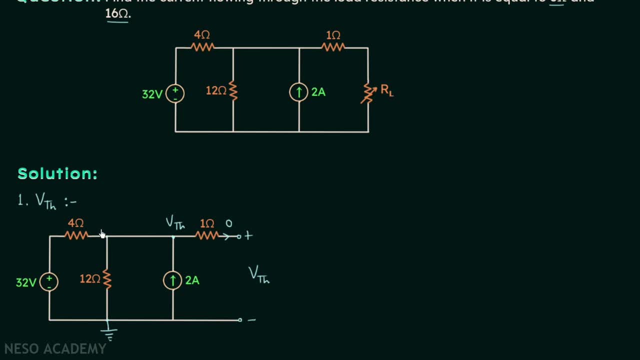 And therefore, if we can find out the potential at this node, we can have Vth. And to find out potential at this node we will use nodal analysis. This is our reference node and this is our principal node And let's say the potential at principal node is equal to Vx. 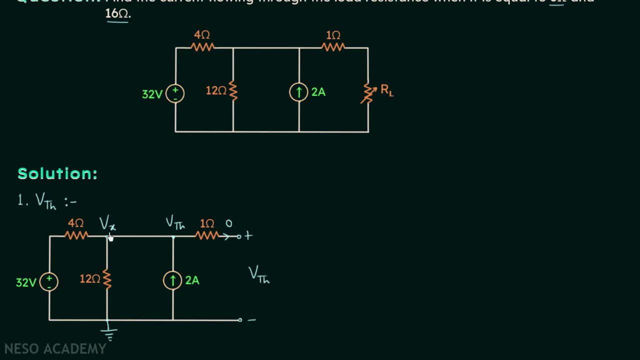 And we know, we assume the potential at principal node to be the largest potential in the network. Therefore, all the currents in the branches connected to this node will leave this node. Let's say this is our current. Let's say this is our current. 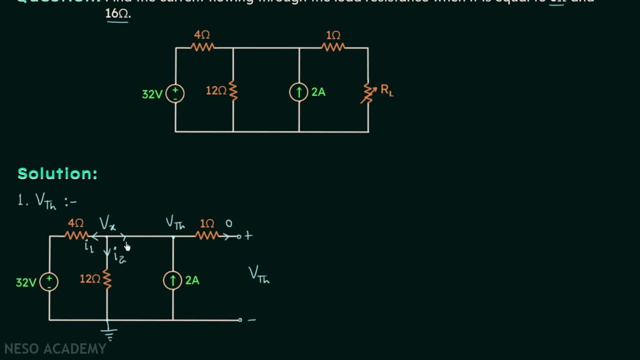 Let's say: this is our current I1, this is current I2 and this one here is current I3.. Now, from KCL, we will have I1 plus I2 plus I3, equal to zero. To find out I1, we need the potential at this node, which will be 32 volts. 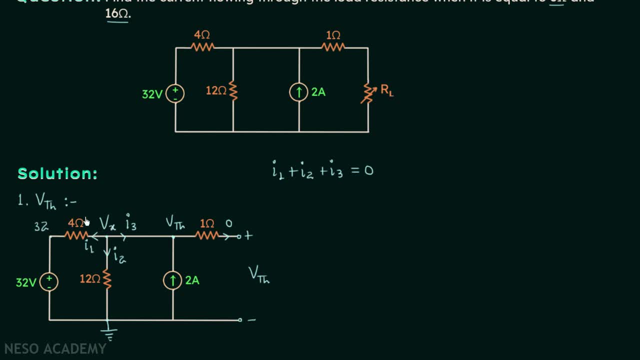 And I1, it will be equal to Vx minus 32 divided by 4.. Then we have plus I2.. I2: it will be equal to Vx minus zero, Zero, divided by 12. So we have Vx divided by 12.. 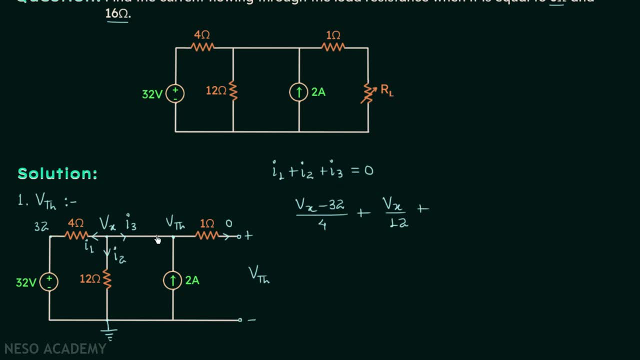 Then we have plus I3.. I3 will flow like this. This means I3 is the current moving in this direction, in this branch, and it is opposite to the direction of 2A current flow. Therefore, we will have I3 equal to minus 2.. 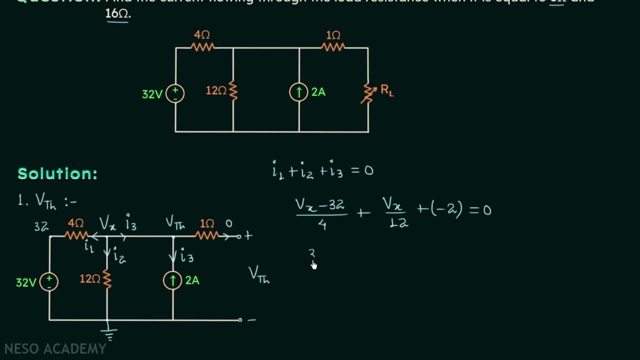 Now doing some rearrangements here. We will have 3 times Vx minus 96, plus Vx equal to 24.. In the next step we will simplify this further. We will have 4 Vx equal to 120.. Therefore, Vx is equal to 120 divided by 4, which is 30 volts. 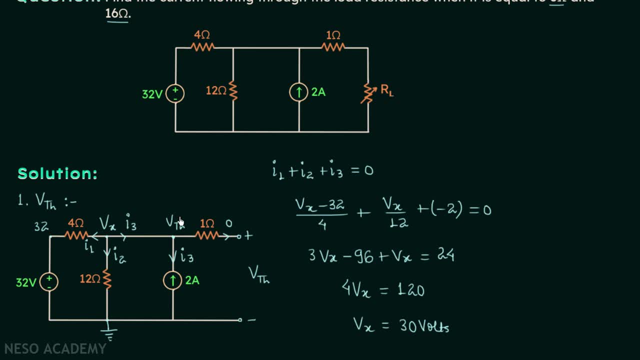 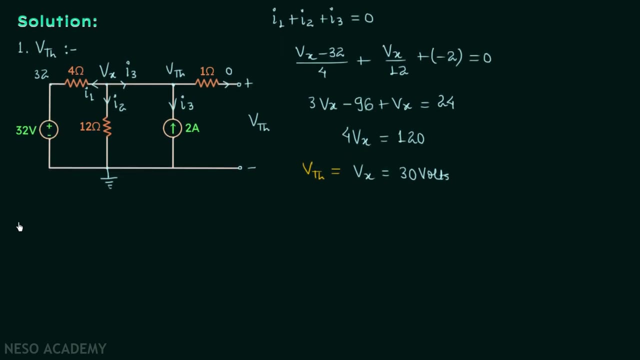 In this way we have obtained the Thevenin's voltage Vth is equal to Vx. Therefore Thevenin's voltage Vth is equal to 30 volts. Now we will move on to the calculation of Thevenin's equivalent resistance. 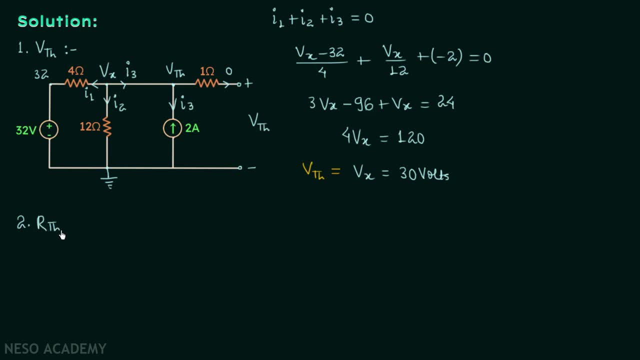 And to calculate Rth. we will do some modifications in our network And the modification number one is Same Modification We did calculating vth. we will open circuit the load resistance and the modification number two is turning off all the independent sources. this is our first independent source. we will turn it off. 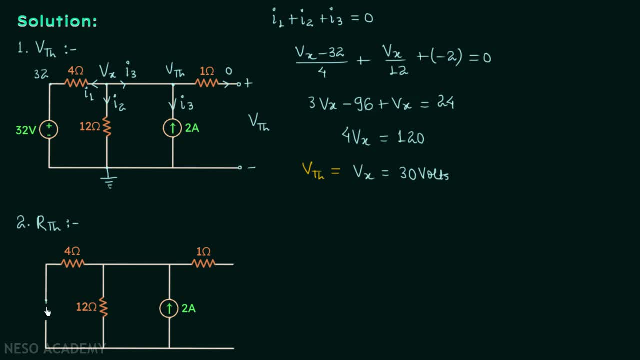 by replacing it with a short circuit like this- and this is our second independent source- and we will turn it off by replacing it with an open circuit- and then we will calculate the equivalent resistance between the two terminals when looked from the side- and this equivalent resistance is known as rth, the thevenin's equivalent resistance- and when you observe the modified 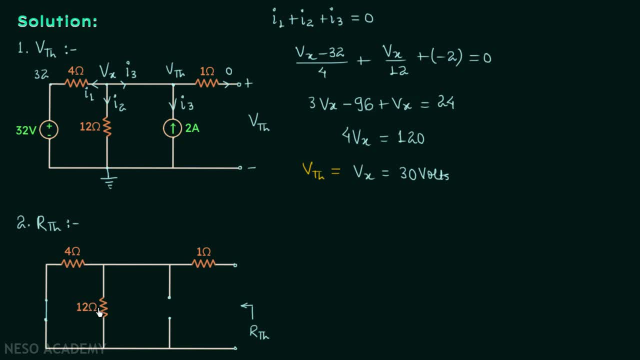 network you will find 4 ohms resistor and 12 ohms resistor. they are in parallel, so rth it will be equal to four, parallel with 12 and their equivalent. their equivalent is then in series with one ohm resistor, so we will have plus one. from here we will have rth equal. 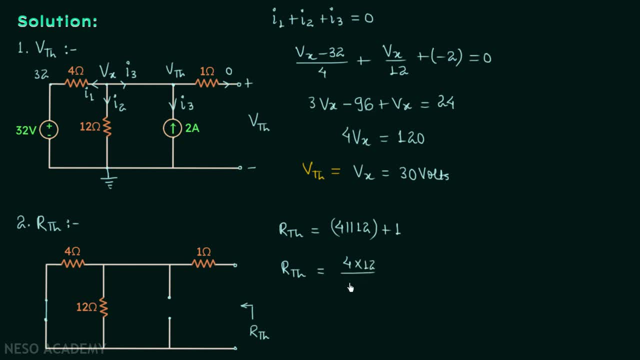 to 4, multiplied to 12, divided by 4 plus 12 plus 1, when you solve it, you will have rth equal to 4 ohms. so in this way we have calculated the Thevenin's equivalent resistance, and we already calculated the Thevenin's voltage, and therefore now we can have the Thevenin's equivalent circuit. 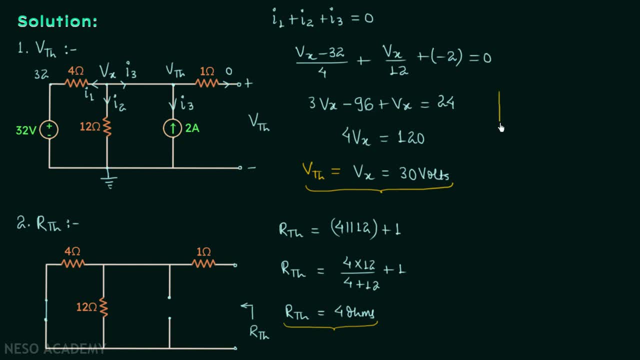 so the circuit will have the Thevenin's voltage, which is equal to 30V, which is connected in series with the Thevenin's resistance, which is 4Ω, and we will have them connected to our load resistance. so this circuit is our Thevenin's equivalent circuit and with the 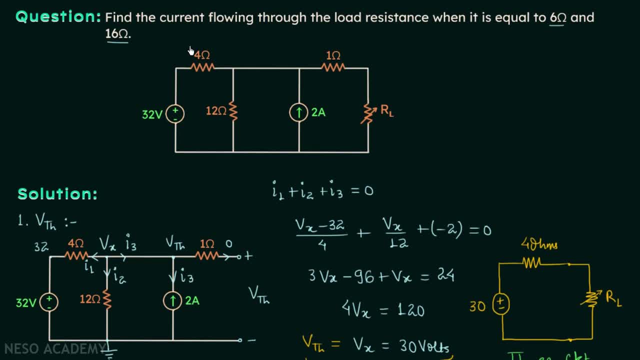 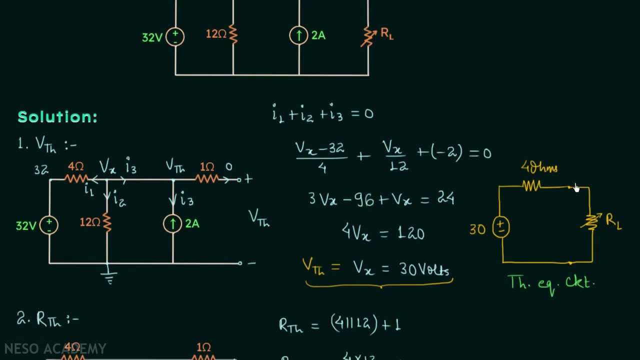 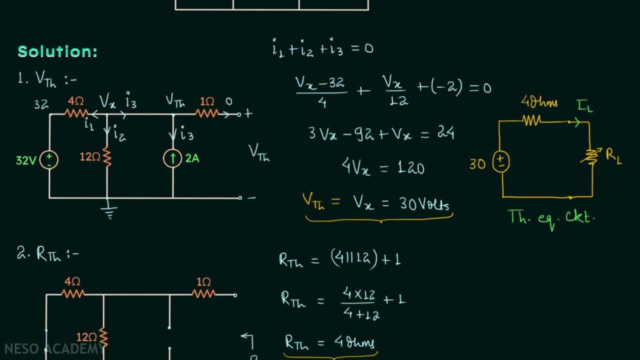 help of this equivalent circuit we are required to find current flowing through RL when it is 6Ω and 16Ω. so first we will assume the current flowing through RL to be I sub L and in case number 1.. When RL is equal to 6Ω, we will have IL equal to 30V divided by 4 plus RL, which is 6.. 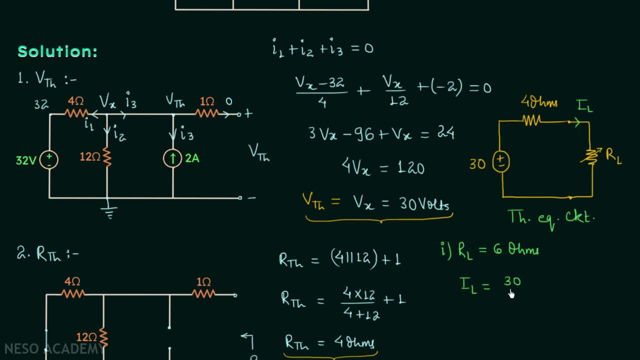 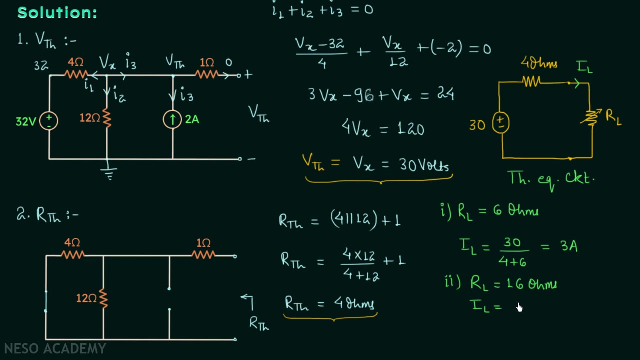 So IL is equal to 30 divided by 4 plus 6. so we have 3A in case number 2.. When RL is equal to 16Ω, IL will be equal to 30 divided by 4 plus 16, 30 divided by 4 plus 16. this will give us: